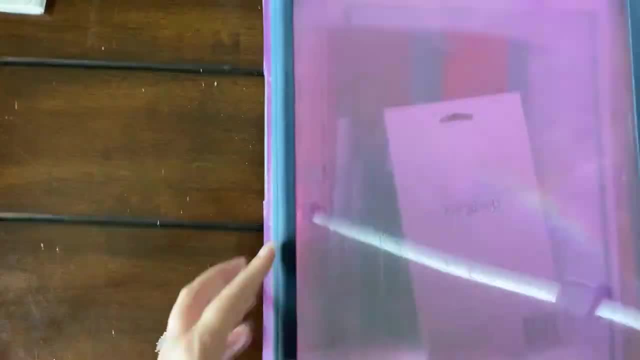 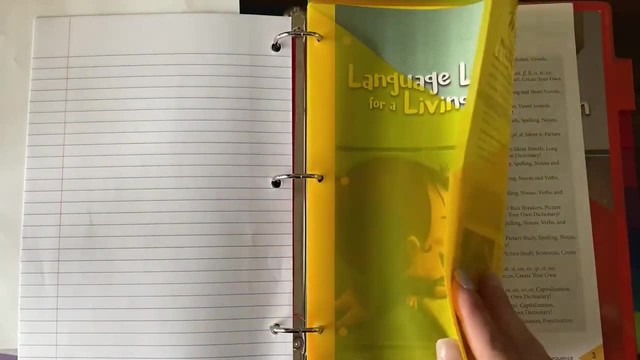 So I have put together an entire binder of stuff just for me which I wasn't really intending to show in this video. Okay, so I made a tab just for the Language Lessons, 1 teacher stuff. So the scope and sequence, It will all be bound in the book already, but since I had them cut the binding. 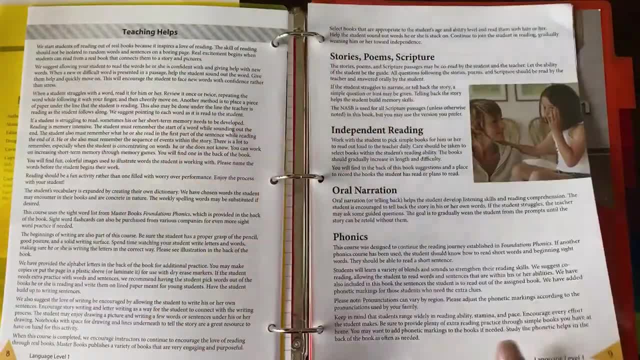 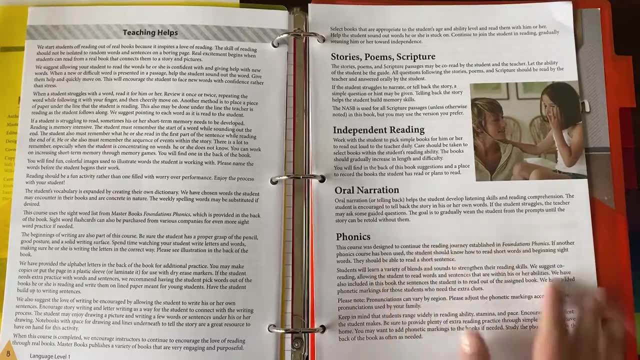 to take all these things off so I could put them right into my teacher's manual. that's where they are. So this front of the book tells you: there's aural narration, there's phonics, practice, independent reading, So lots of scripture. There's spelling and creating your own dictionary. 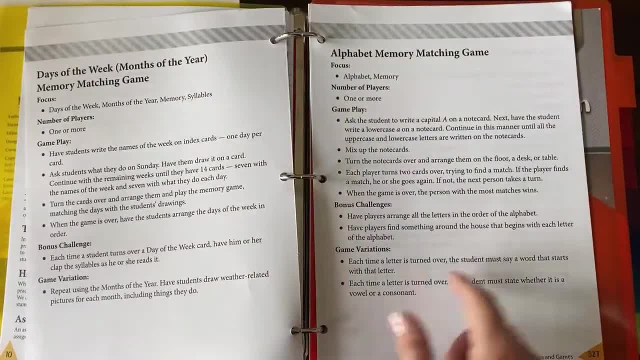 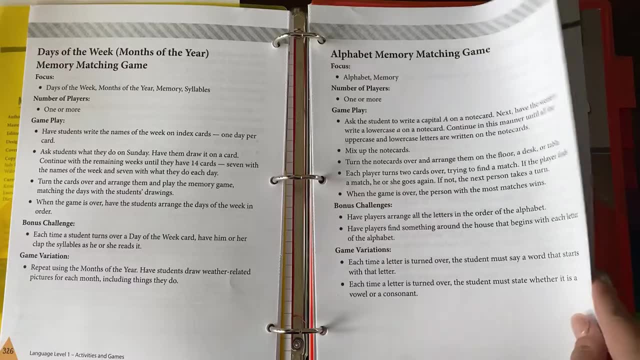 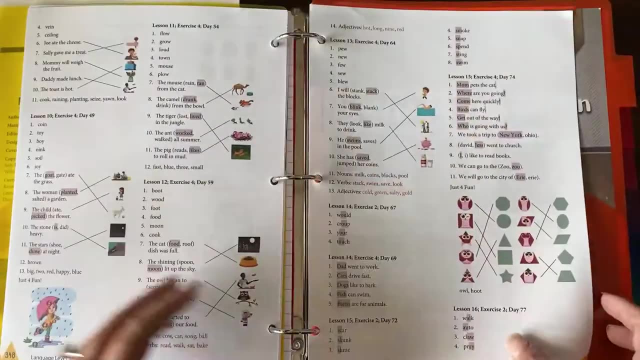 And there are all kinds of supplements and activity ideas for the teacher. These will actually be. Do you notice the page number here? These are actually in the back of that book. So, and then there's answer keys here, As if I need help with first grade answers. but I suppose 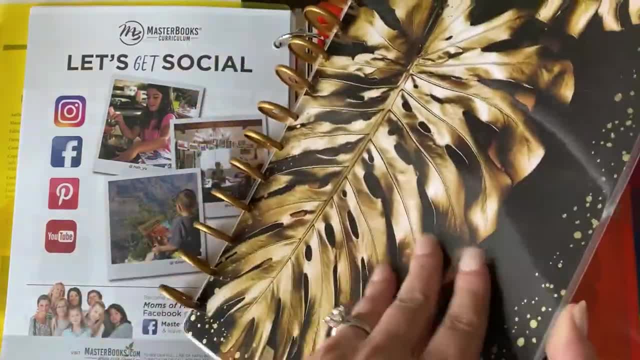 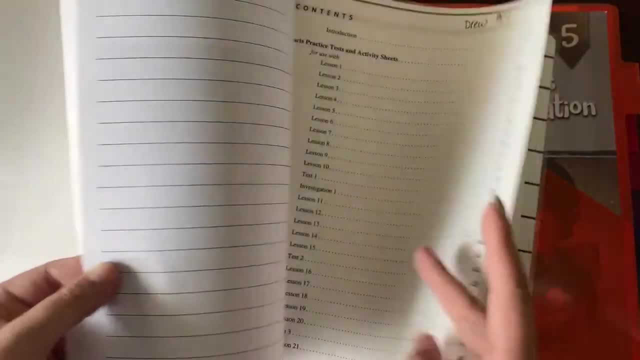 suppose there is a chance, And then I'm making myself a second kind of binder where I can keep track of their progress. So all of the scope and sequences for all of my children's work throughout the year. This is how I'm going to do it, Instead of writing a lesson plan as they do the work. 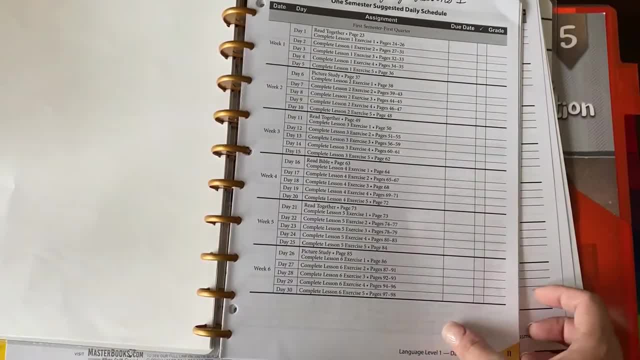 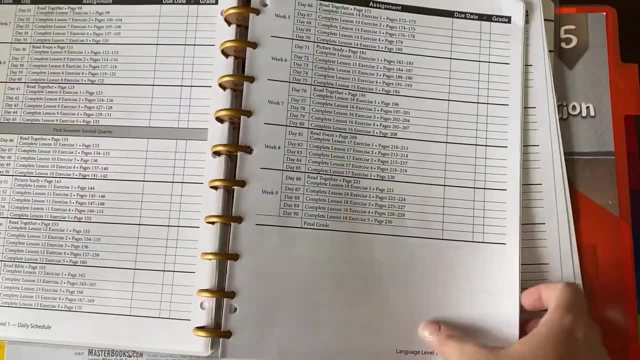 I'm just gonna check it off here and that's how I'm gonna know what kind of progress we're making. So they do give you these lesson ideas. This is for five days a week. We'll see how that goes. Let's see They've got. 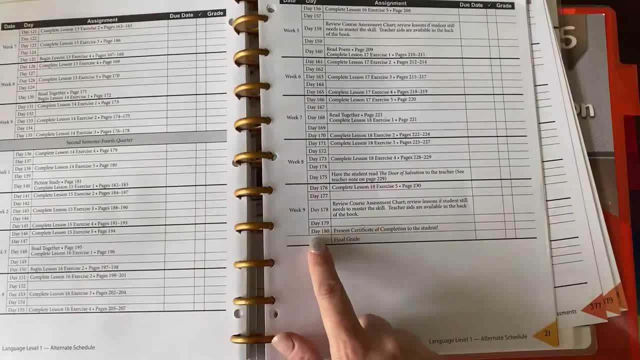 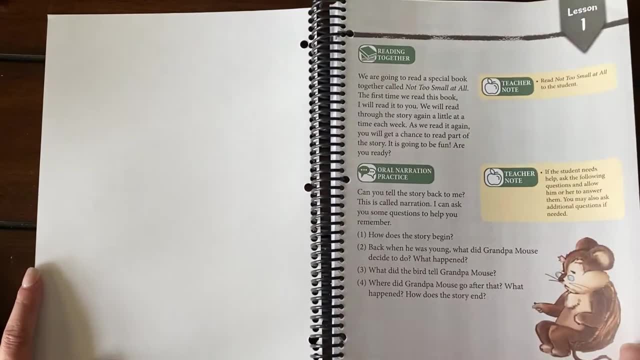 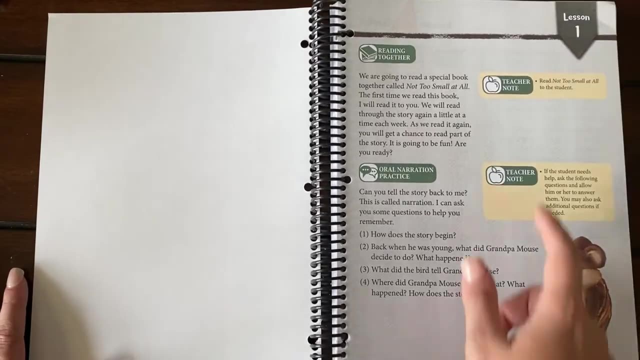 two semesters worth of work. There is a hundred and eighty days of work in this book. Okay, so lesson one: There is some talking about what we're gonna do this lesson, some oral narration. How does the story begin? So we're reading from: Not Too Small at all. 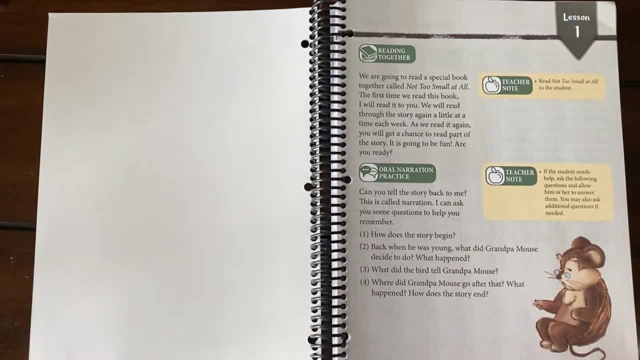 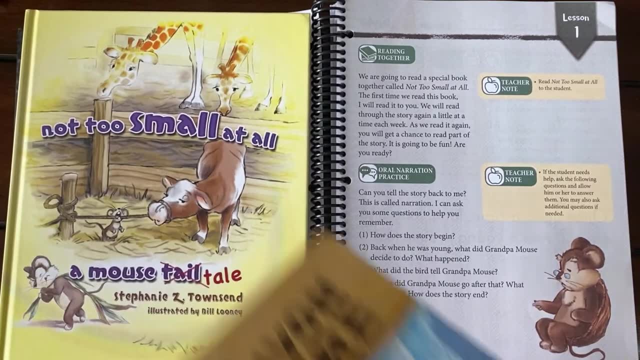 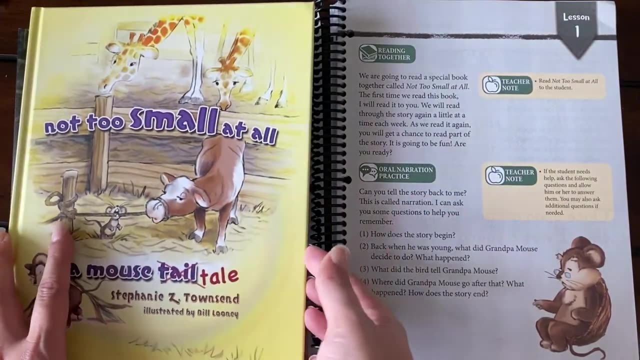 So there are some supplemental books that you are also supposed to purchase with this curriculum. There's the Door of Salvation by Ken Ham, Here's the Not Too Small book And the Grand Canyon Adventure. So I purchased those separately, So it looks like lesson one We're gonna be starting out in this book. 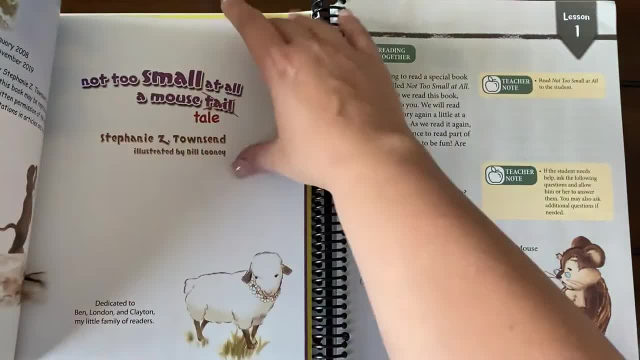 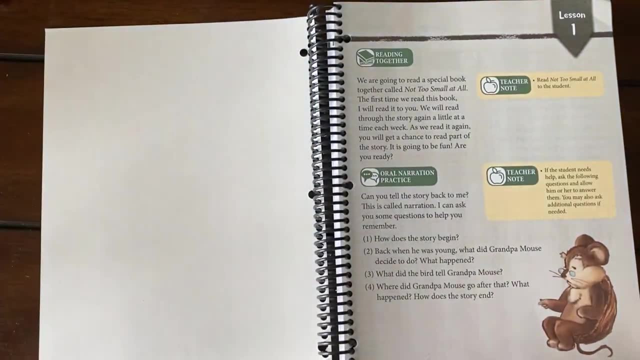 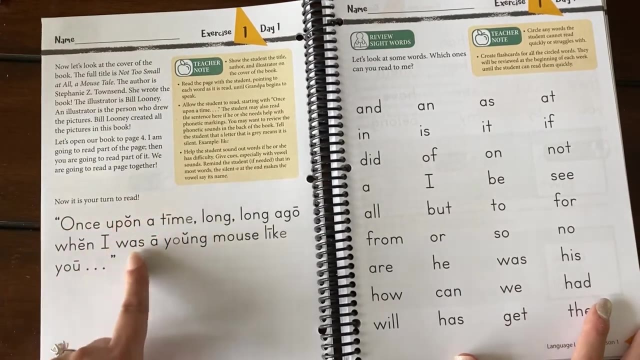 We're gonna be reading about it- Sorry, reading from the book, Not Too Small at all- And then she's gonna answer some questions about it. We'll be in that book for several lessons And then she's going to be learning how to read and reading these little symbols to help decipher what the words are. 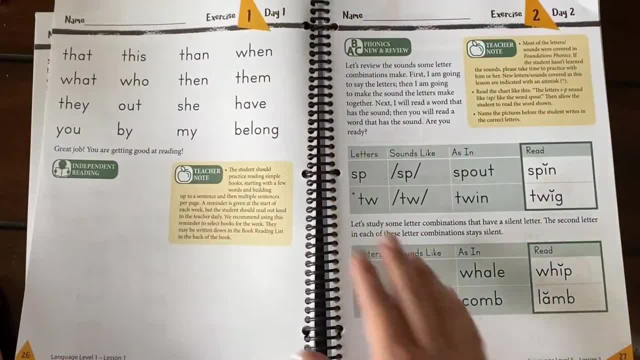 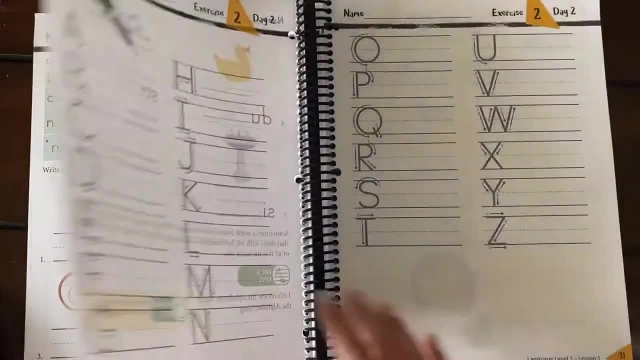 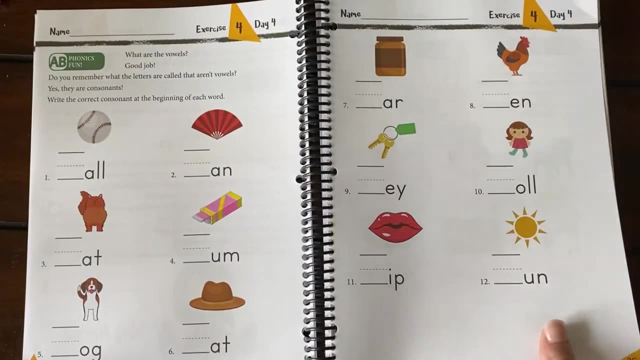 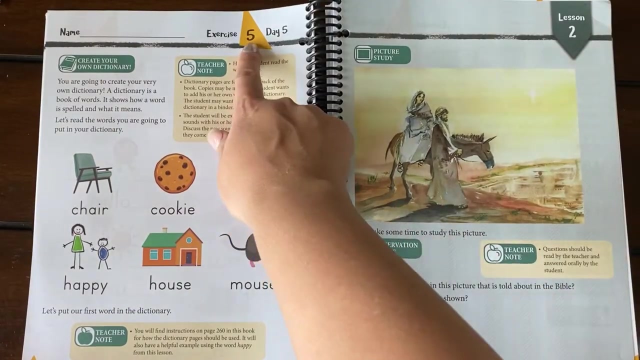 Taking a quiz, what she already knows: reviewing sight words, some phonics practice in here and then some worksheets type the printing practice. my daughter's gonna be doing a formal printing curriculum from the good and the beautiful in addition to this. okay, and then we've got lesson two. so see, this is day five. this is what else I 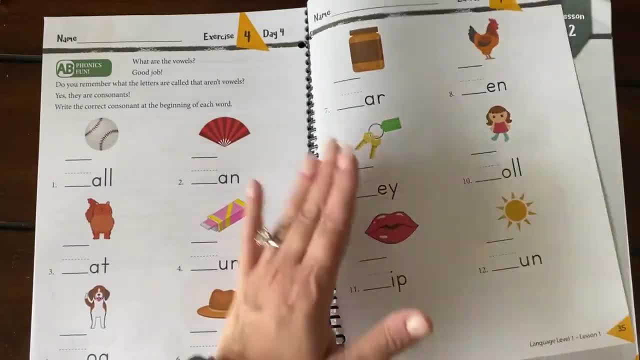 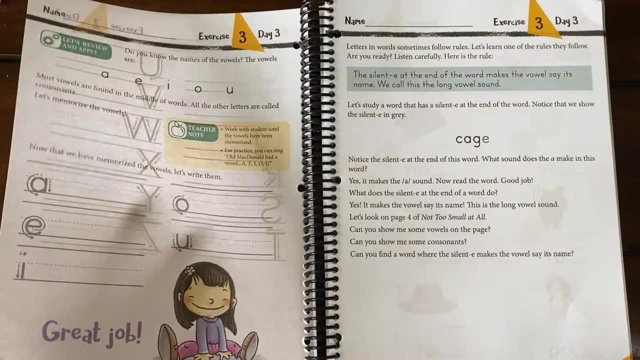 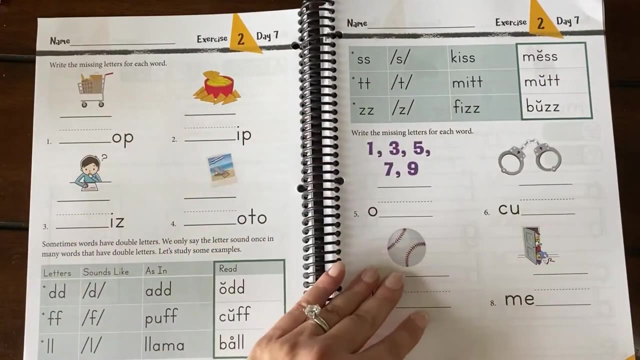 should have pointed out. a little itty-bitty lessons per day. so day four worksheet right here. this is it day three, not very long at all. so if you have a child with a short attention span, this is great. if you have a child who is thirsting for more, like my child is, then just add to it. there's all kinds of 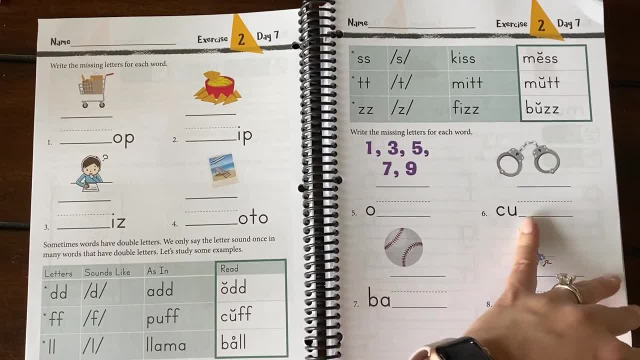 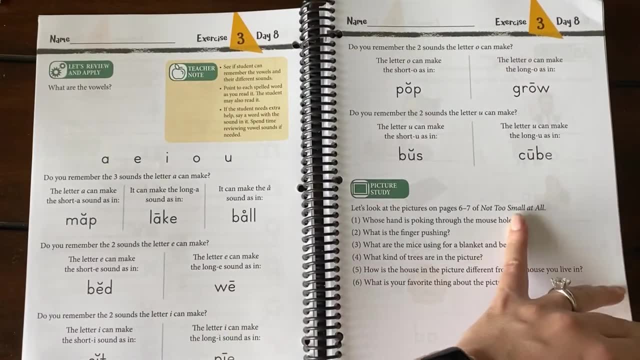 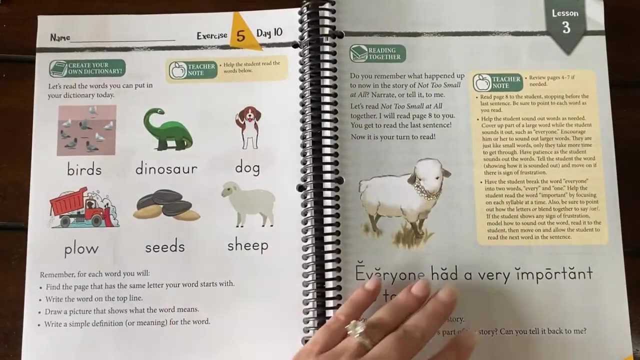 things you can do here. I've also got some phonics cards so we can practice our phonics- flashcards from another curriculum I've used in the past. we're gonna be doing a lot of independent reading, reading aloud. we have some a Becca readers. I have tried the Becca kindergarten program before and I didn't finish it. 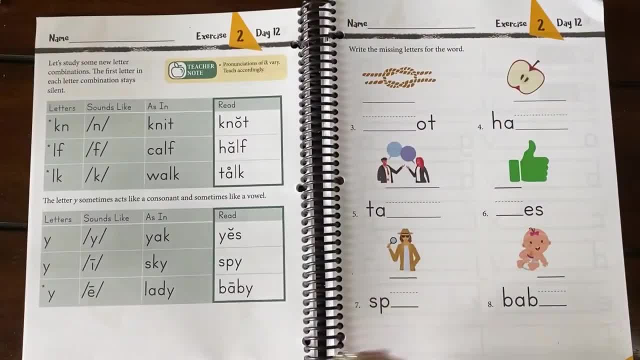 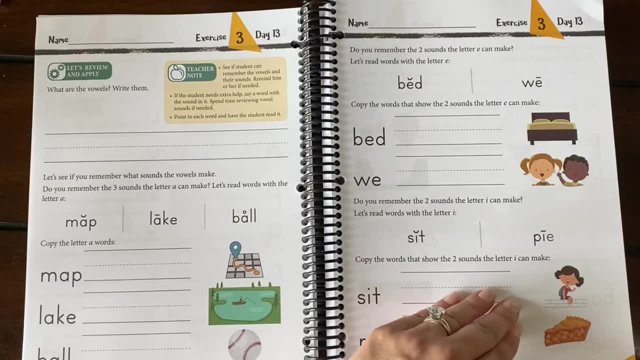 with my second child. so I still have all those worksheets. if my child this one, if this isn't enough for her, then I will just pull out those old former at the work sheets and she can just go to town. so this is what it looks like from. 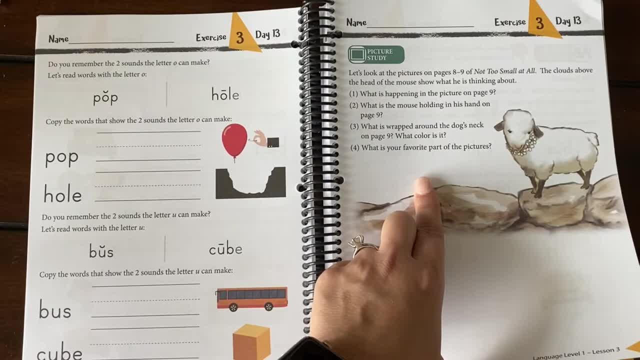 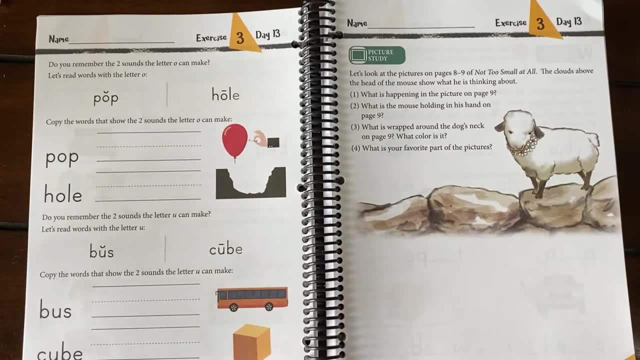 lesson to lesson. lesson three we've got. let's look at the picture from. it's not too small at all. on page nine. the clouds above the head of the mouse show what he's thinking about, what is happening in the picture on page nine. so let me just 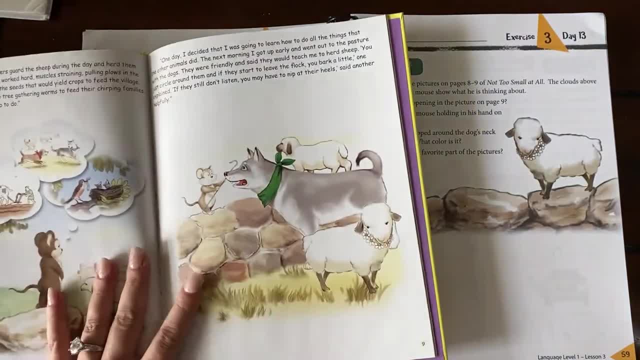 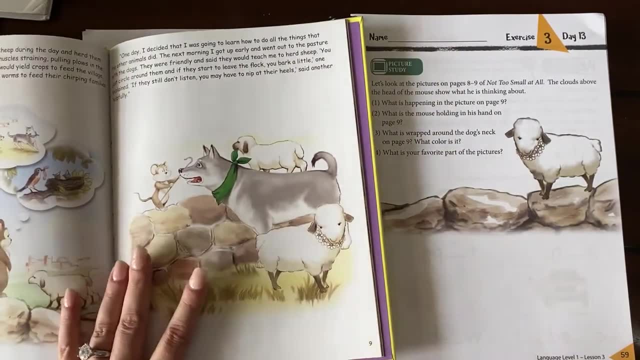 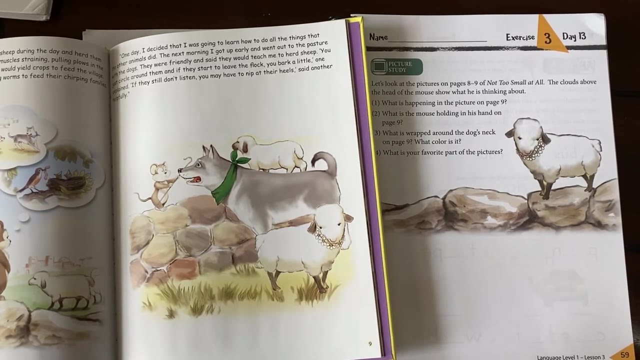 show you an example of that activity. so here's the pages we'll be focusing about. so this tells you what he's thinking about. so what's happening on page nine? and so then she'll be answering whatever she thinks. what is the mouse holding in his hand on page nine? this is great dialogue between us, just a fun way to engage with. 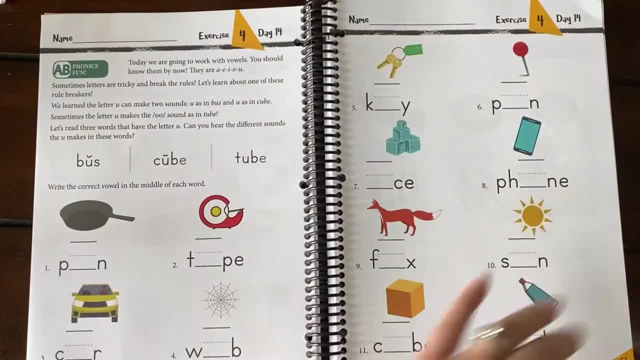 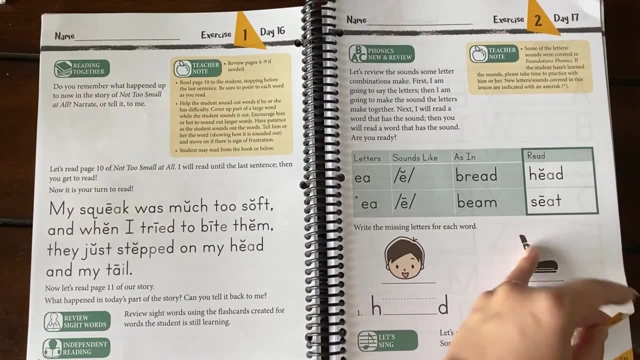 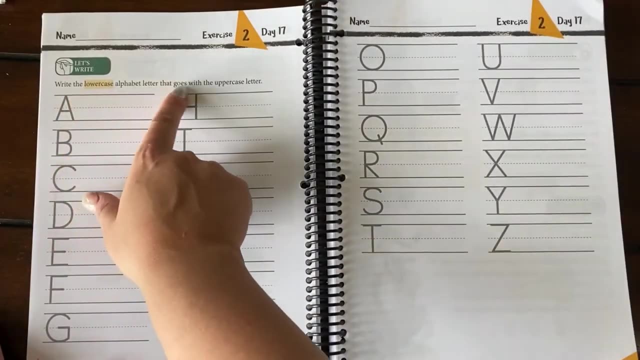 your child. some good prompts on there, thinking about what bells exercise. day one for lesson 16, I think it just I'm flipping through multiple pages here. some more printing practice. this says: write the lowercase alphabet letter. that goes with the uppercase. day three is just the sheet. let's see if you remember what sounds. 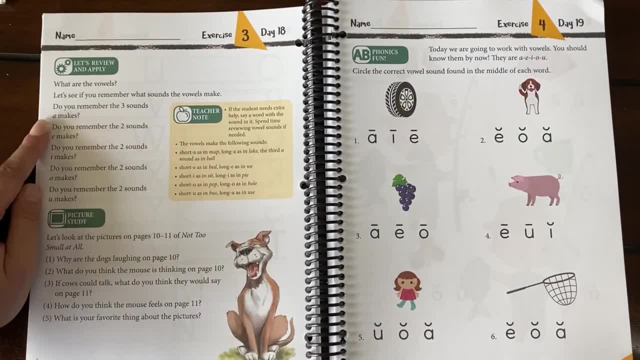 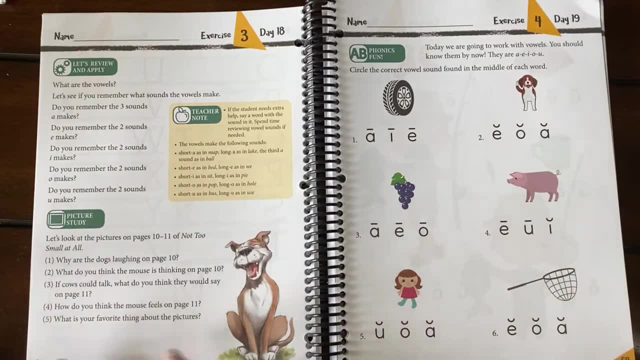 the vows me do you make? do you remember the three sounds? a makes a. do you remember the two sounds he makes? do you remember the two sounds I make? so this will be good practice. another picture study: let's look at the pictures on page 10 and 11 of not too small at all. 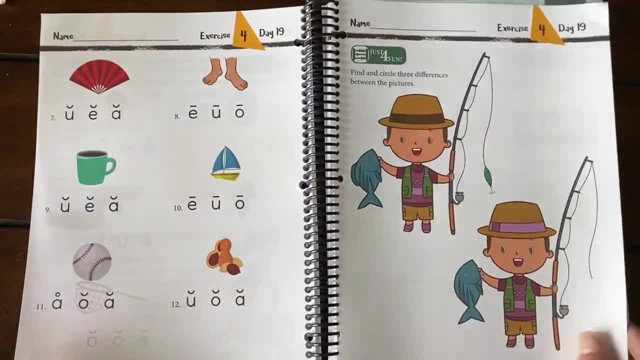 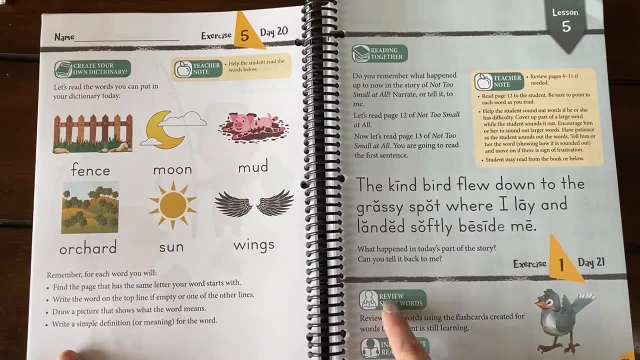 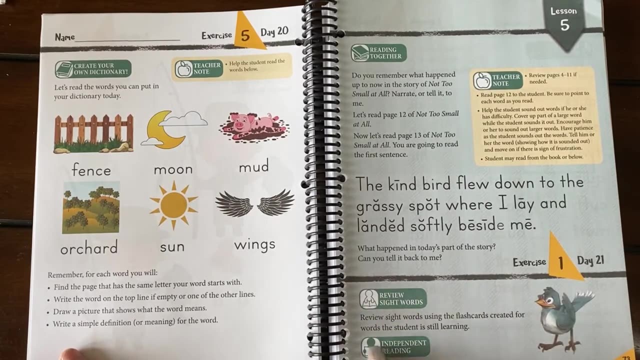 day four, work day four. day four: find the differences between the pictures. and then day five, and so on and so forth. and then there's these little teachers notes here to tell you what you're gonna be doing. review little prompts to remind you, review your sight words. also, don't forget the independent reading phonics. 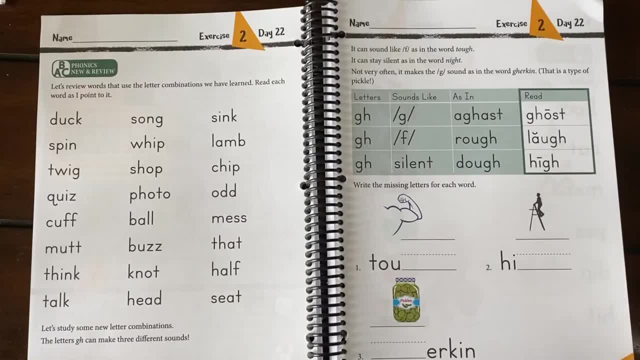 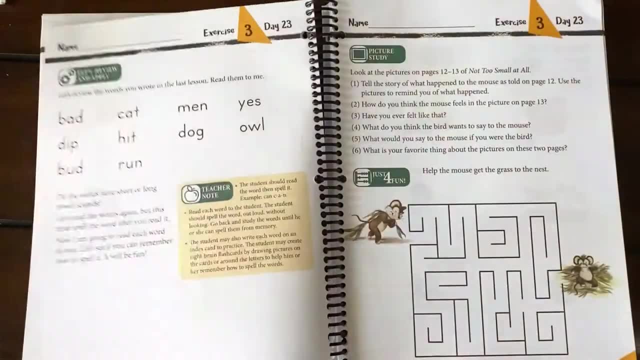 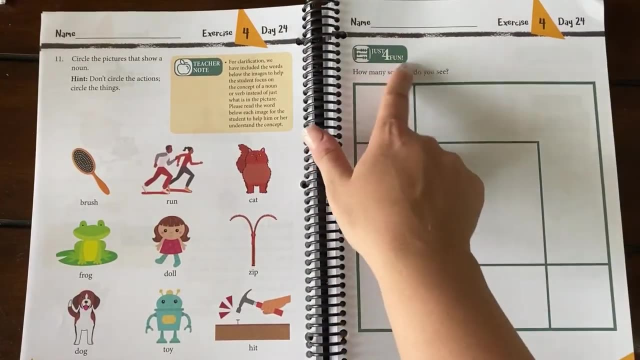 new and review. so if you make, you might want to make some flashcards for your child, things that they need to remember. that's what those teachers tips that I showed you in my other binder would show you. so this is it just for fun? how many squares do you see? this one's tricky one? 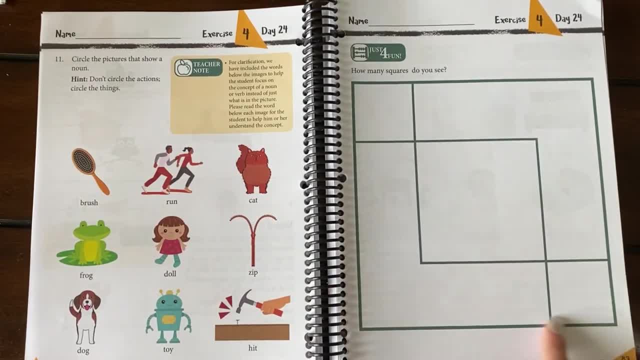 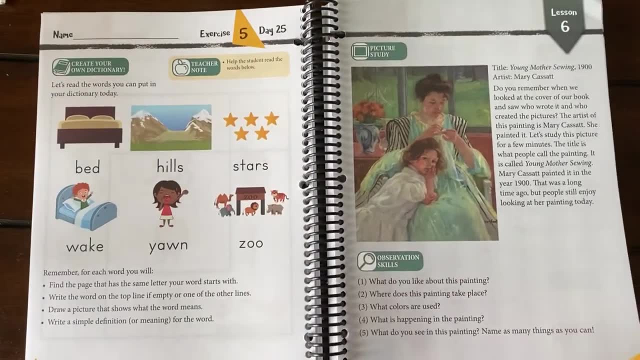 two, three, four, five, six. let's see how astute your child is and teaching them how to be observant. another picture study. so this is a picture study that's actually good because it's built for kids, but it is also for kids. it's nice to. 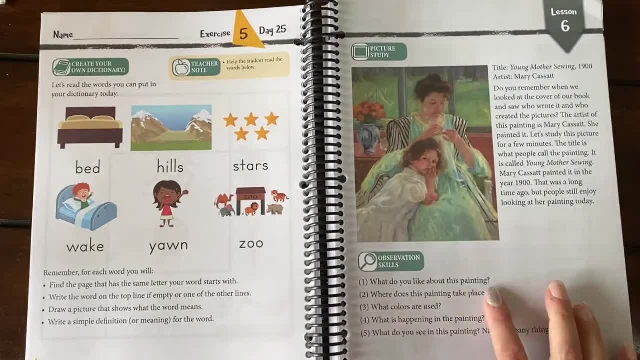 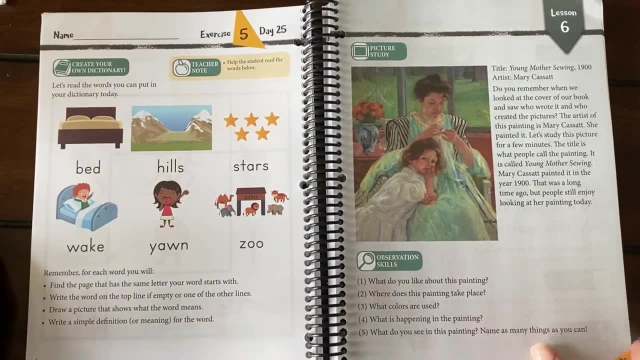 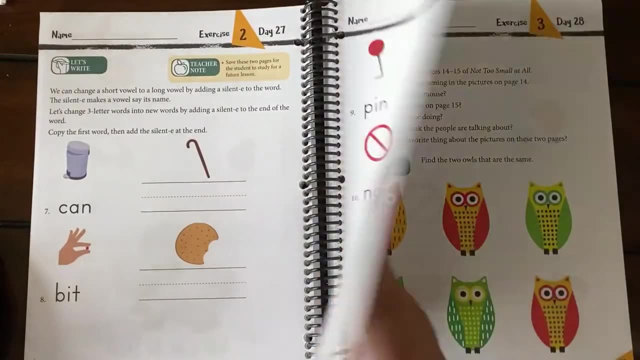 be more of an advertising art course. so let's see a picture study from a famous painting, so not from the not too small book, so that's thrown in there also. what do you like about this painting? where does this painting take place? so the child is using their imagination. now what's happening in the painting? and 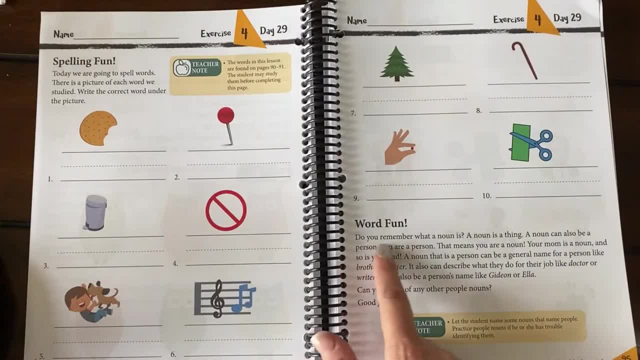 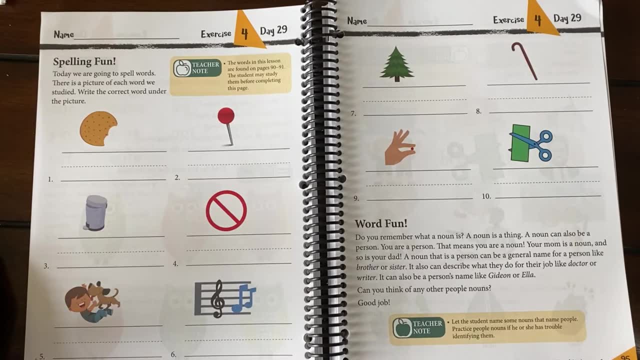 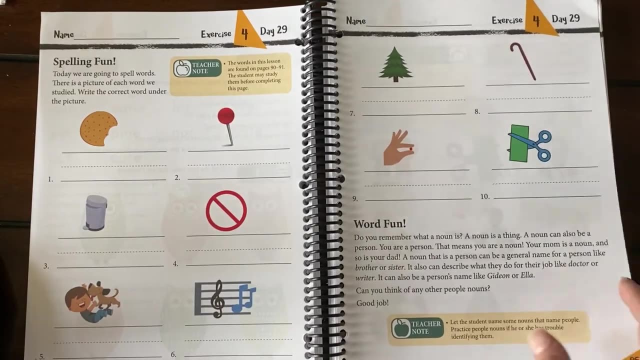 stuff, word, fun. do you remember what a noun is? a noun is a thing, so my daughter would. a noun names a person, place, thing, activity or idea from classical conversations. but that's why it's fun, when you've done other curriculums too, to see what they remember. 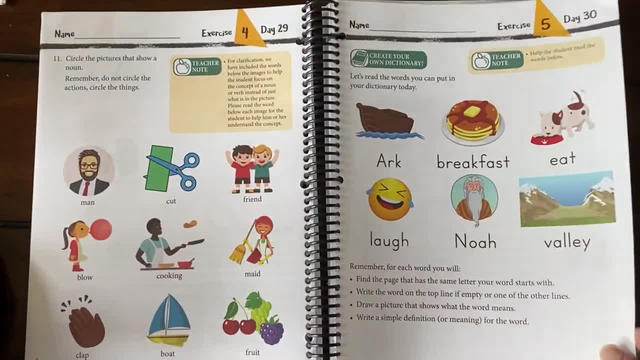 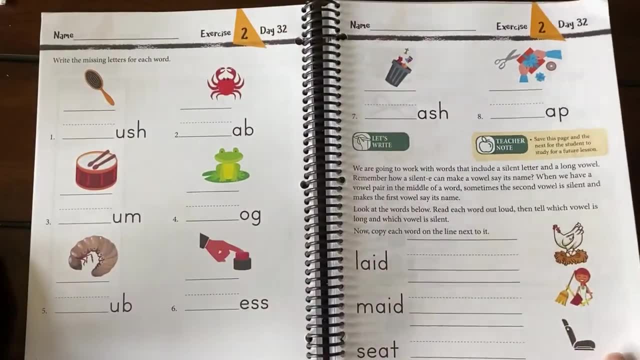 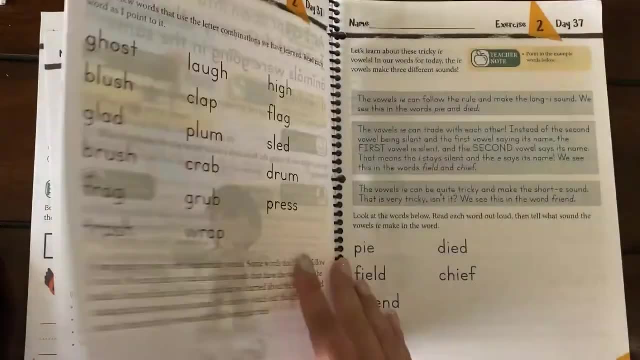 I don't remember learning about a noun when I was in first grade, though, so maybe that's because it was so long ago. So this is basically it In a nutshell. this is the new language lessons for a living education First grade. you could probably do this in kindergarten.